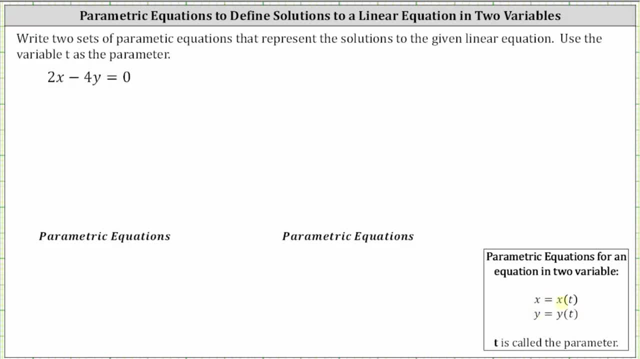 the given linear equation. To do this, it'll be helpful to solve the given equation for x or y. In this case, we'll do both, so that we can have two sets of parametric equations that represent these solutions. Let's first solve the given equation for x. 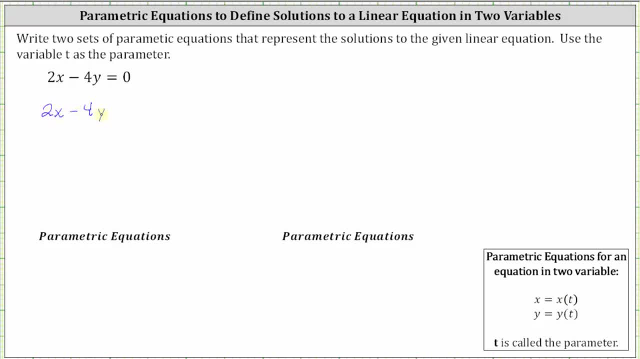 So, beginning with two x minus four y equals zero. to solve for x, we would first add four y to both sides, which gives us two x equals four y, and then divide both sides by two. Simplifying, we're going to have x equals two y. 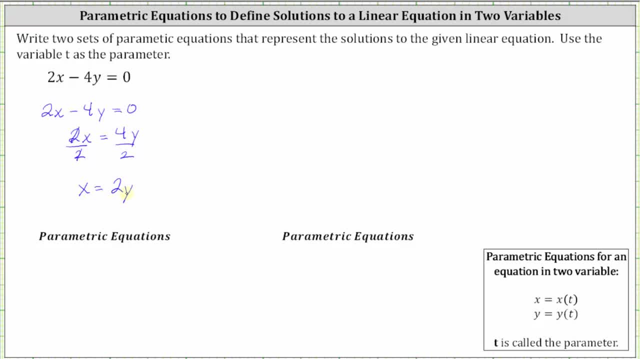 Now that we have the equation solved for x, to write the parametric equations, the easiest thing to do is to let y equal t. So if we let y equal t be one of the parametric equations, if y is equal to t, notice x is going to be equal to two times t. 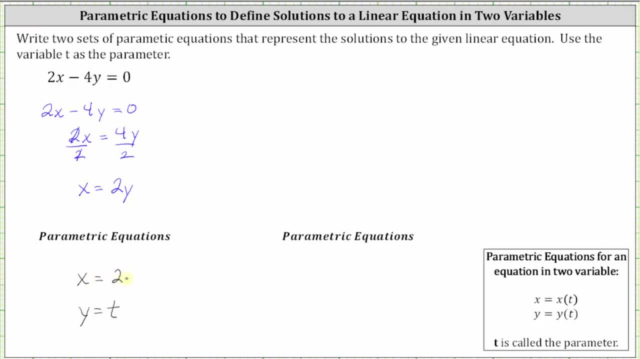 or x equals two t, And now we have parametric equations that represent the solutions to the given linear equation. So in this form, for any value of t, the outputs of x and y will satisfy the given linear equation. To get the second set of parametric equations, 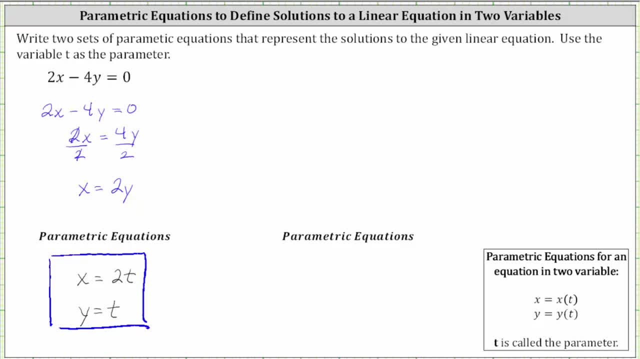 let's solve the same equation for y. We could just divide x equals two, y by two on both sides to solve for y. But let's go ahead and start over with the original equation: Fract two x on both sides. 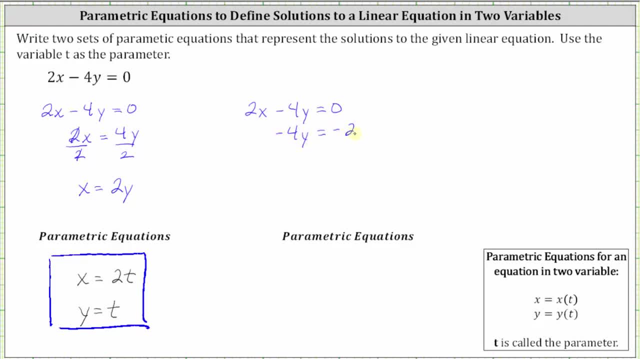 which gives us negative four. y equals negative two, x, and then divide both sides by negative four, Simplifying we have y equals on the right. negative two divided by negative four simplifies the positive 1 1⁄2,, giving us y equals 1 1⁄2 x. 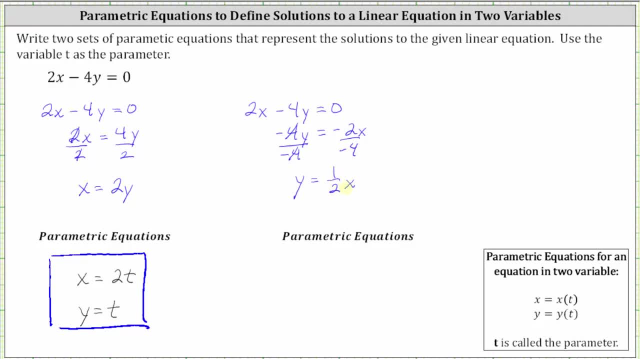 Here because we have the equation solved for y. the easiest way to write the parametric equations would be to let x equal t. Notice: if x is equal to t, then y is equal to 1 1⁄2 times t, or y equals 1 1⁄2 t. 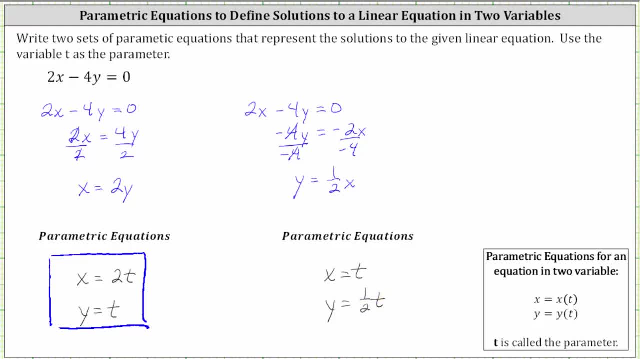 These parametric equations also represent the solutions to the given linear equation. Before we go, let's take a look at a graph of the original equation as well as the parametric equations. In blue we have the graph of the original linear equation. 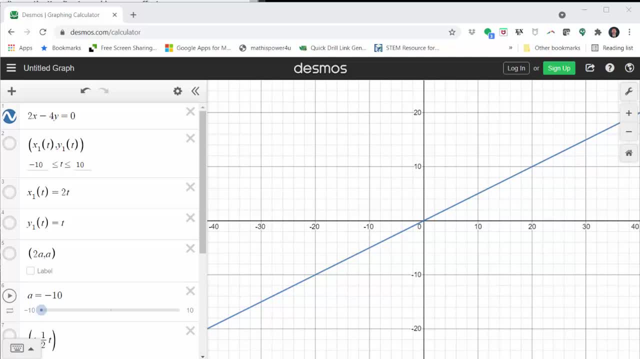 two x minus four y equals zero. Remember, in this form the lines do go in both directions forever. And now let's take a look at the graph of the parametric equations: x equals two, t and y equals t. Typically when graphing parametric equations, 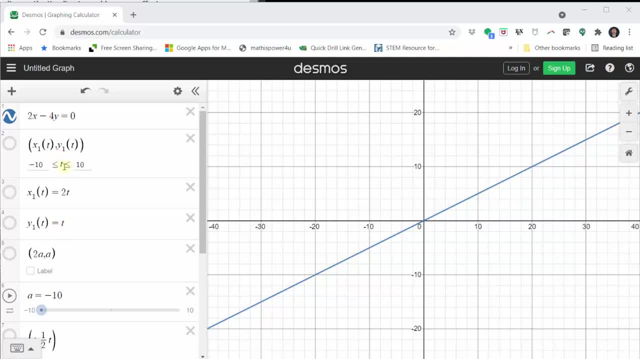 we define an interval for t. Here we have the closed interval for t from negative 10 to positive 10.. So because we have a specific interval for t, it's not going to graph the entire line. If I turn this on, we can see the parametric equations. 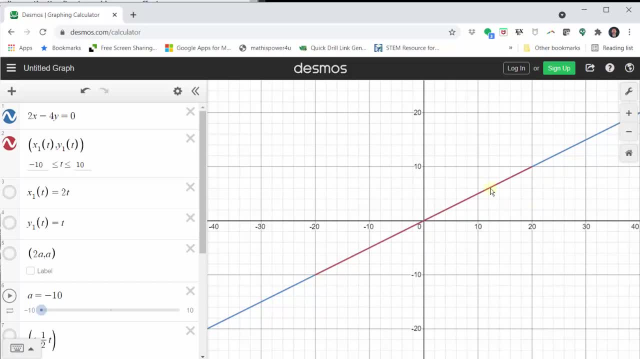 and the resulting graph here in red. Notice how it's only graphing it in red. It's only graphing a piece of the line, which is actually a segment. So as we change the interval for t, it would change how much of the line is graphed. 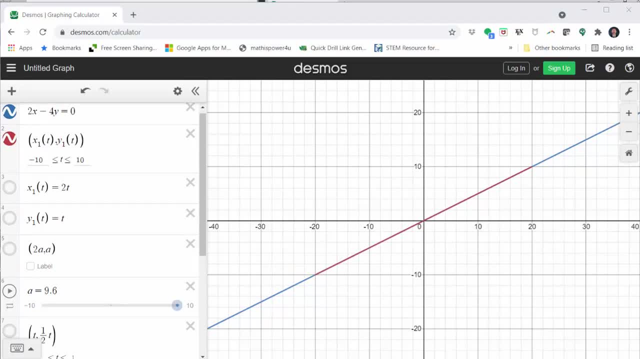 If we did let t equal all real numbers, then the red line would be exactly the same as the blue line. Also, notice how all of the points on the red segment are on the blue line and therefore we know our parametric equations are giving us solutions to the original linear equation. 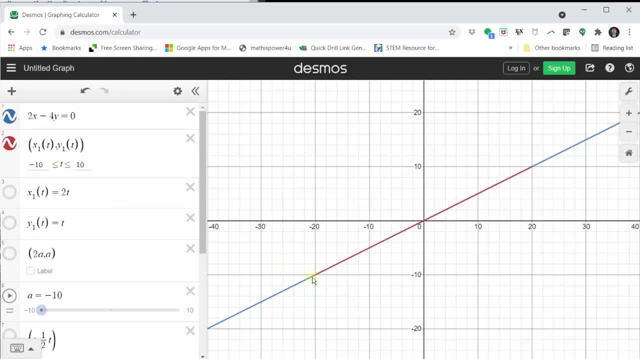 If we think of t as time, we can think of the red segment being traced out in a particular direction, which is called the orientation of the graph given by the parametric equations. So to show this, I'm going to go ahead and turn on the point 2a, comma a. 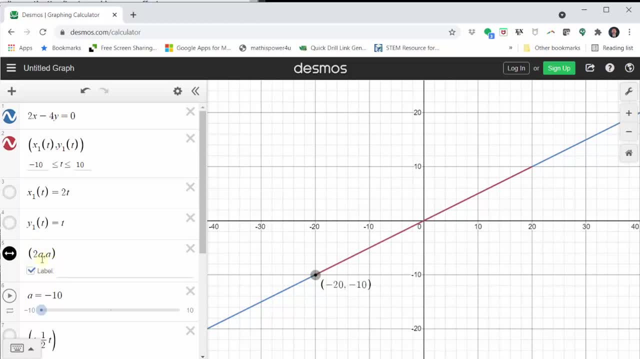 and then change the values of a, which represent the parametric equations. Notice, when t is negative 10,, the x value is negative 20, and the y value is negative 10.. And as t increases from negative 10 to positive 10,. 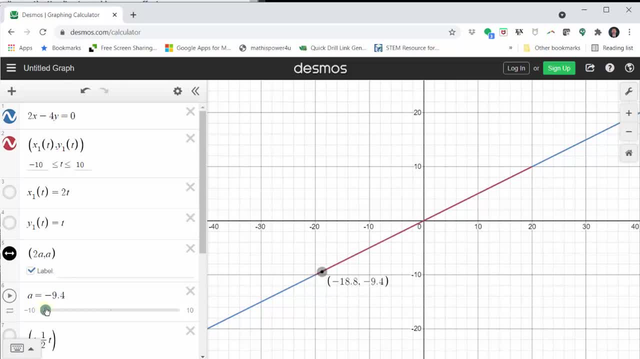 we can see the direction in which the line segment is being traced out, So you can think of this as a way to animate a point along a particular path, using parametric equations. Again, each of these points are on the red line as well as the blue line.